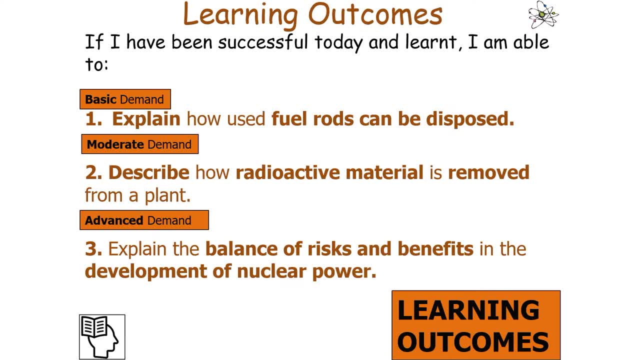 and learnt in today's lesson. we should be able to explain how fuel rods can be disposed of, describe how radioactive material is removed from a plant and then finally explain the balance of risks and benefits in the development of nuclear power. So we're going to be covering the following. 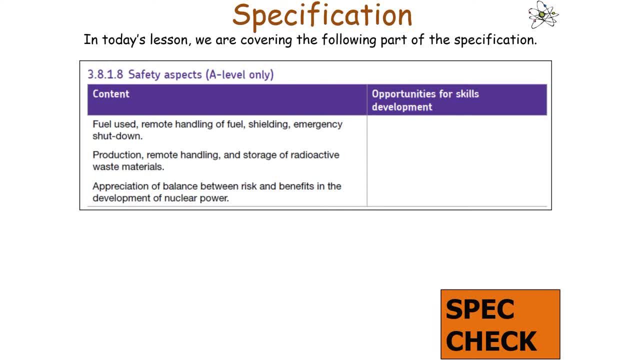 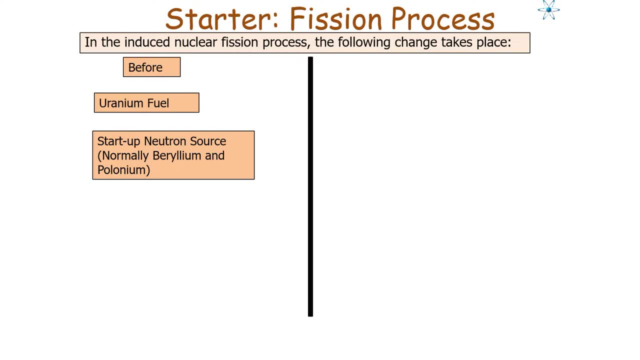 part of the AQA A Level Physics specification 3.8.1.8, safety aspects. So in an induced nuclear fission process the following change takes place: Beforehand you've got a uranium fuel and a start up neutron source, so either normally beryllium or polonium. Then after the fission process you'll 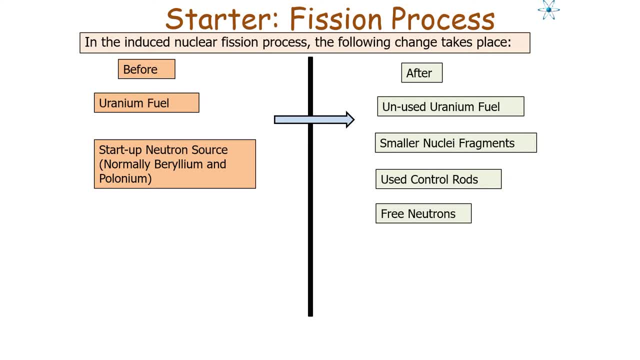 have some unused uranium fuel, smaller nuclei fragments from the fission process itself, used controller rods and free neutrons and in addition to this you'll have energy released as kinetic energy of the products due to the mass defect. Now the material afterwards is commonly 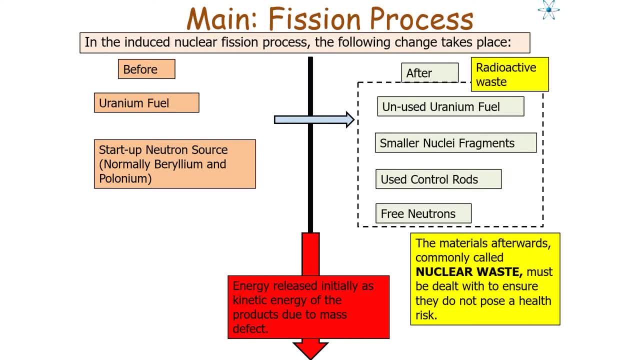 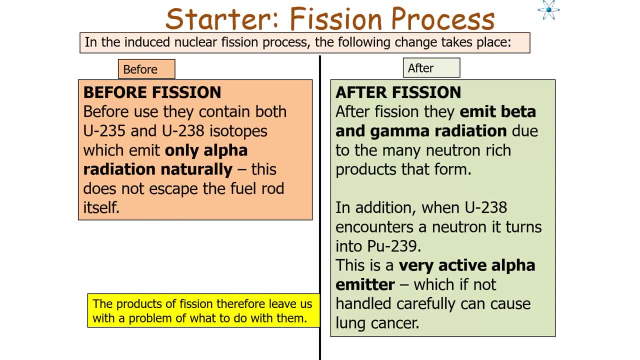 called nuclear or radioactive waste, and it must be dealt with to ensure that it doesn't pose a health risk to the humans or the environment around it. So if we think of the following: before the fission process you've got uranium-235 and uranium-238 isotopes. Now both these isotopes only. 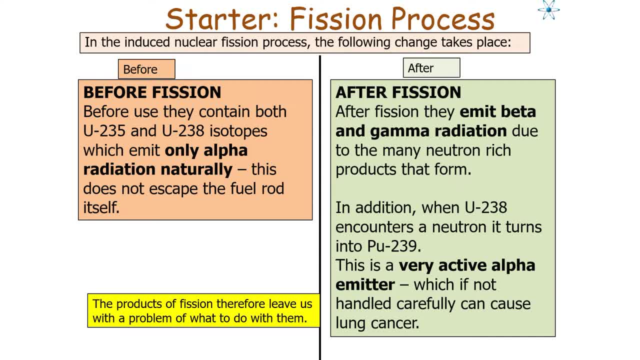 emit oxygen In the fission process, you're going to find that the nuclear fission will emit alpha radiation naturally. Now this won't actually escape the fuel rod casein, so the the reactants in this particular process are not going to pose a health risk to people in the surrounding environment. 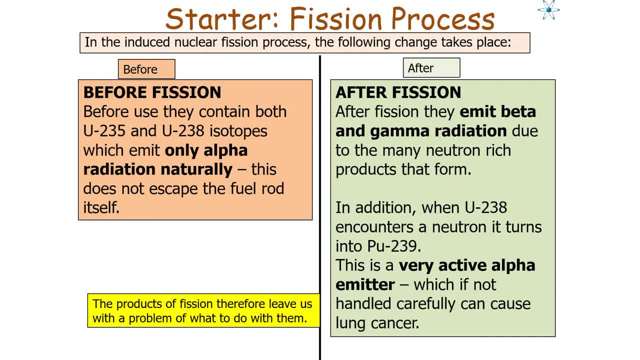 But after fission the fragments of the of the nuclei produced in the fission process will emit beta or gamma radiation. because you tend to find that the products of nuclear fission tend to be very neutron rich in their composition, so are very radioactive. And in addition, in the fission 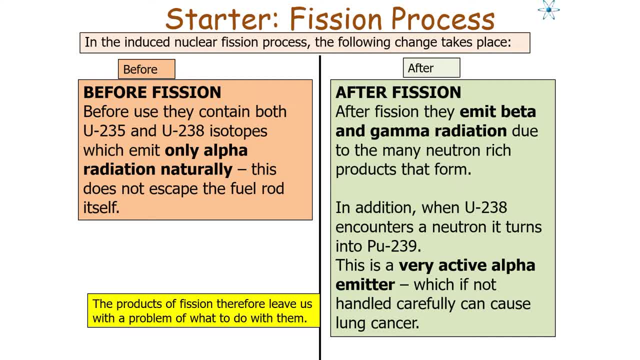 process, you'll have times when uranium-238 encounters a neutron and turns into plutonium-239, which is actually a very active alpha emitter which, if not handled carefully, can actually cause lung cancer. So the products of fission leave us a problem of what to do, not the actual reactants. 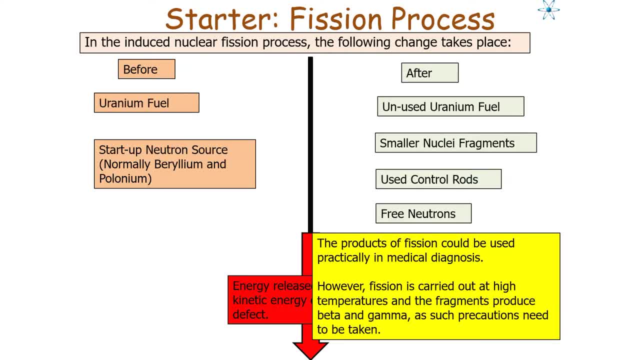 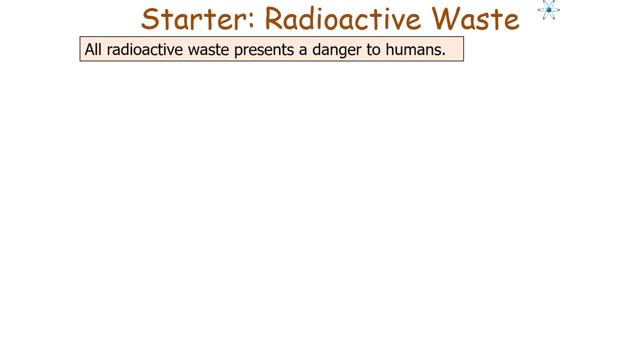 of the fission process. Now the products of fission can be used practically in a medical diagnosis. however, fission is carried out at high temperatures and the fragments produce beta and gamma, so as such precautions need to be taken Now. all radioactive waste presents a danger to humans. This is because 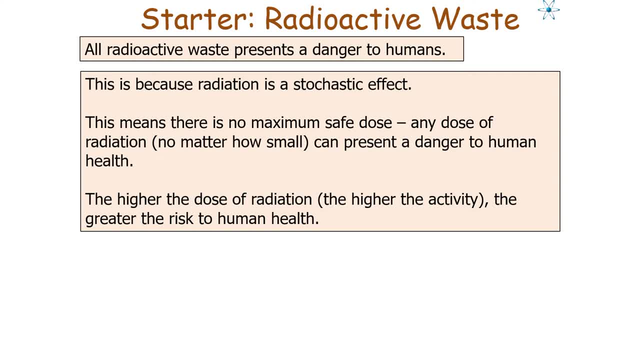 radiation is a stochastic effect. This means there's no maximum safe dose. Any dose of radiation, no matter how small, can present a danger to human health. Now, the higher the dose of radiation, so the higher the activity, the greater the risk to human health. So this leads us to classify. 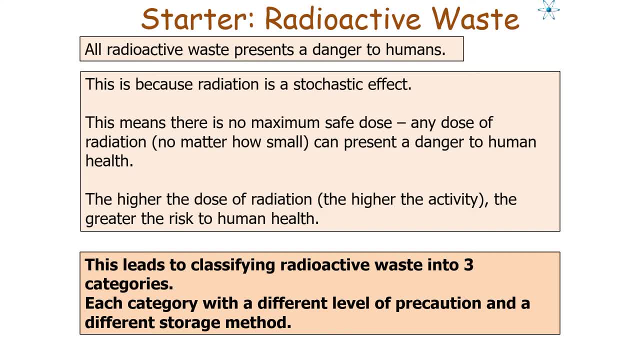 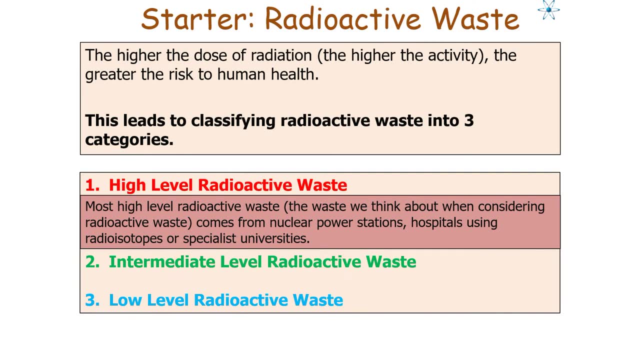 radioactive waste into three categories, Each category with a different level of precaution in different storage method. So you've got high level radioactive waste, intermediate level radioactive waste and low level radioactive waste. Now, most high level radioactive waste, which is the waste we think about when we consider radioactive waste, comes from nuclear power stations, hospitals using 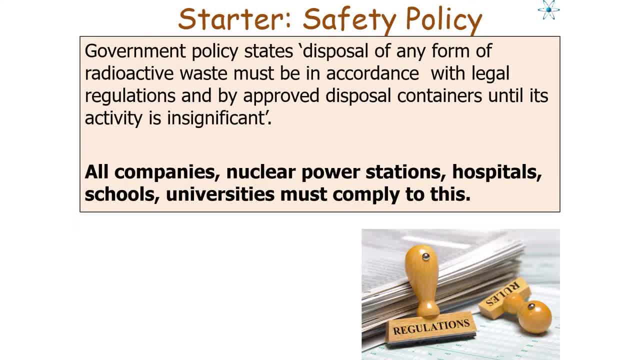 radioisotopes or specialist universities. Now it's important to note that in the UK the government policy states that the disposal of any form of radioactive waste must be in accordance with legal regulations and by approved disposal containers until its activity is insignificant, the same as the background. So all companies 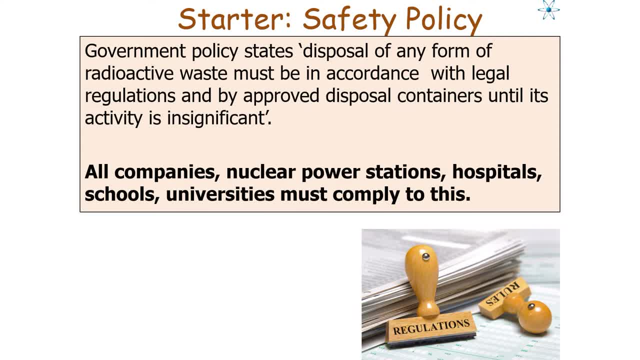 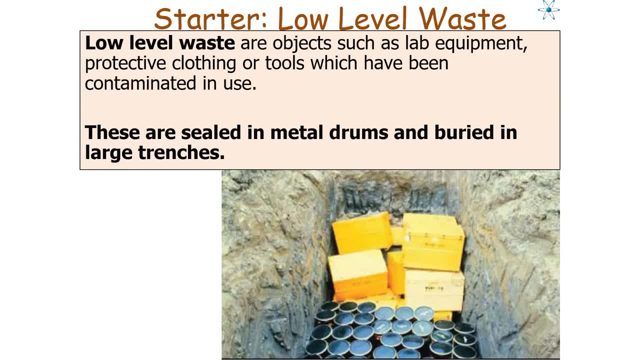 all universities, all schools, all hospitals, all nuclear power stations must comply with this. But how do we dispose of each type of radioactive waste? Well, with low level radioactive waste, which is objects such as lab equipment, protective clothing or tools which have been contaminated in. 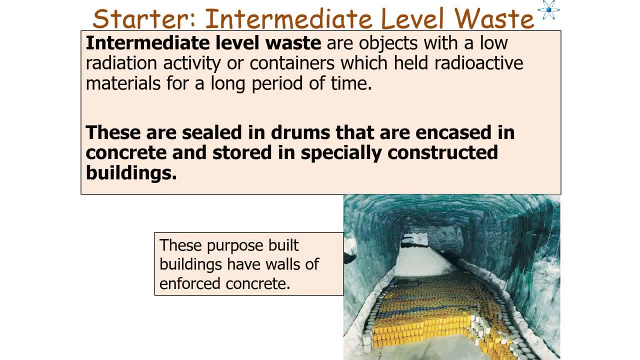 use. they're sealed in metal drums and buried in large trenches. Intermediate level waste are objects with a low radiation activity or conditions such as high radiation activity or conditions such as mm 137.5, which carry radioactive materials for a long period of time. 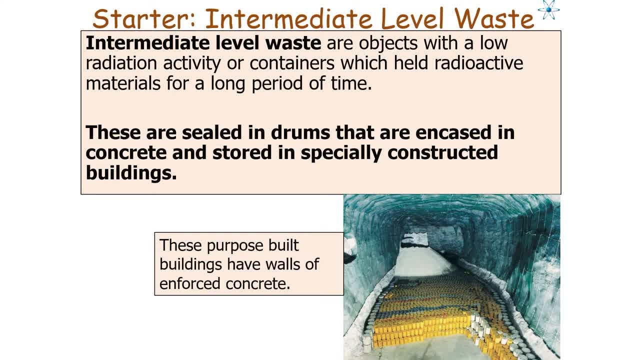 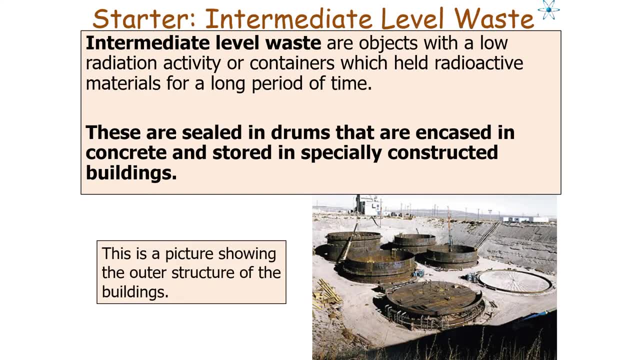 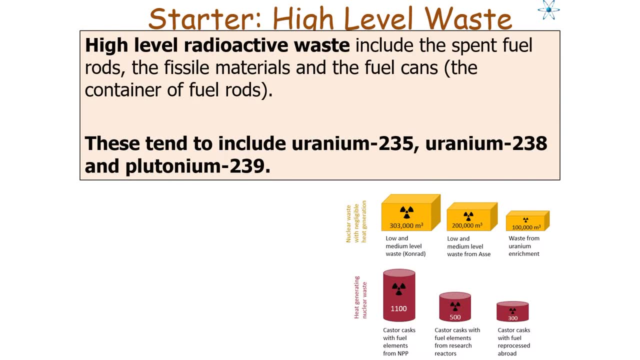 Now this waste is sealed in drums that are encased in concrete and then stored in specially constructed buildings. These purpose built buildings have walls of enforced concrete. Now again, here's a picture showing the outer structure of one of these buildings. Now, high level radioactive waste tends to include the spent fuel rods. 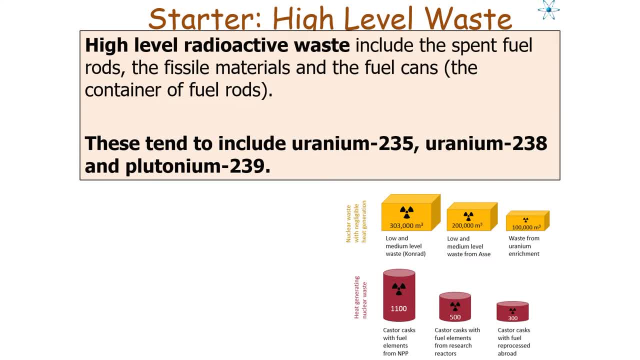 the fissile materials and the fuel cans. what we contain our fuel rods in. This tends to includeoriouroase, migrant, abi olun- handling machinery, Wetopro Kern and plastic lubrication pasette. These containers can fold up the overdrive to allow the CO2 to go out. 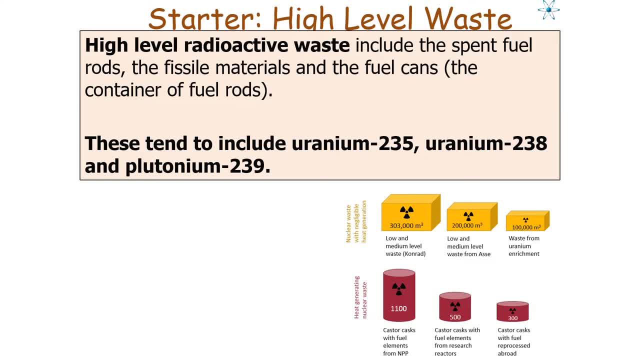 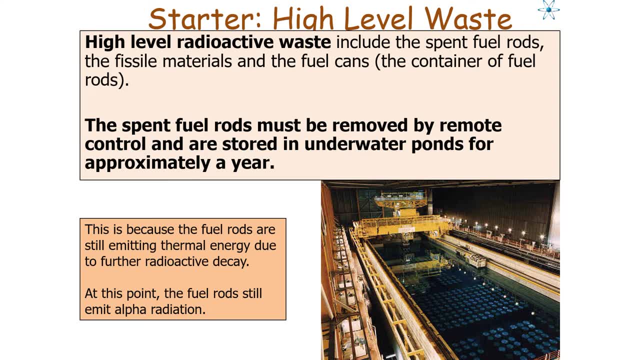 addressed this sp empez vag, america, arriving from final states, tofi for obras de bas smarte, madrid, current uranium-235,, uranium-238 and plutonium-239.. Now it's important to note that what happens is the spent fuel rods are first removed by remote control, so a human doesn't actually handle them at any. 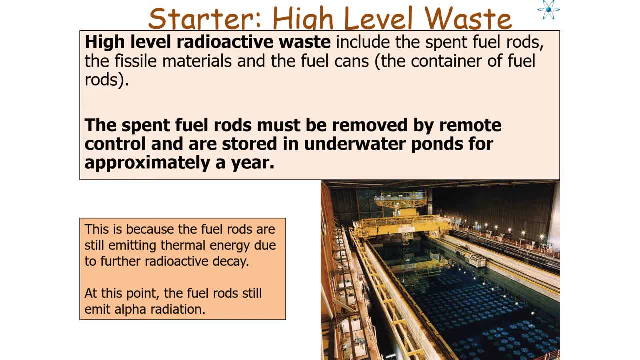 point and they're stored in underwater or cooling ponds for approximately a year. This is because the fuel rods are still emitting thermal energy due to further radioactive decay and the fuel rods are still emitting alpha radiation. So these underwater ponds: firstly, cool the fuel rods down. 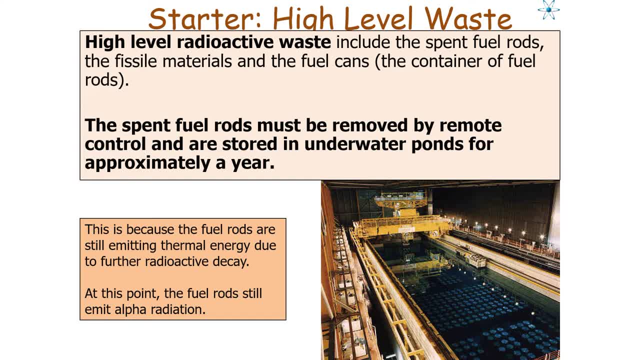 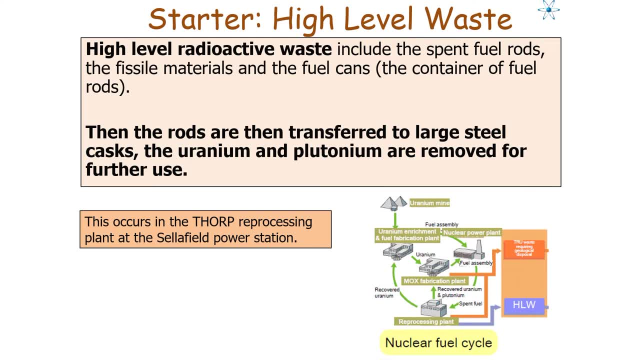 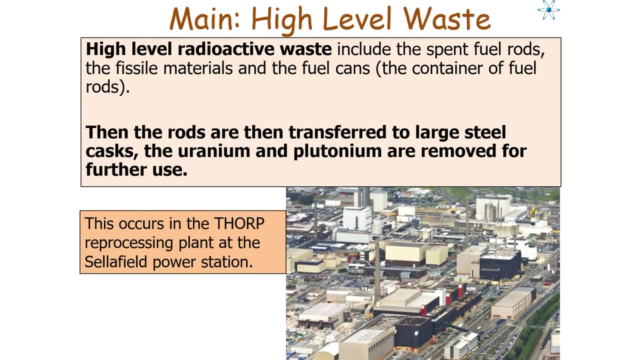 and secondly block any alpha radiation emitted by the fuel rod. Now the fuel rods are then transferred to a large steel cask and the unused uranium and the plutonium are removed for further use. Now in the UK this occurs in the Thorpe reprocessing plant found at the Sellafield power station. Now 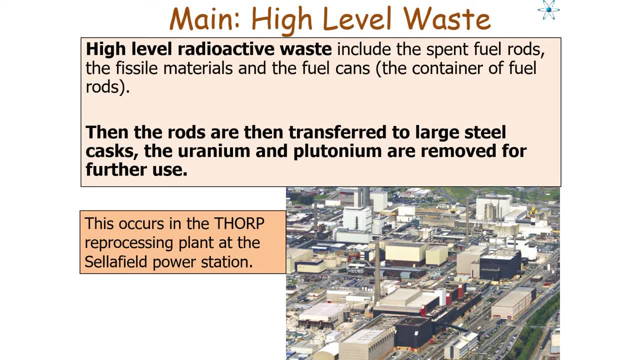 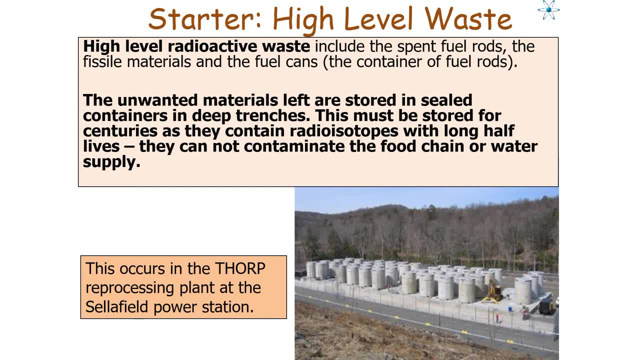 it's important to note that the name of taking the unused uranium and recycling for another fission process is called reprocessing. So you can see here our reprocessing plant. After reprocessing, the unused uranium and plutonium are removed for further use. Now this occurs in the Thorpe. 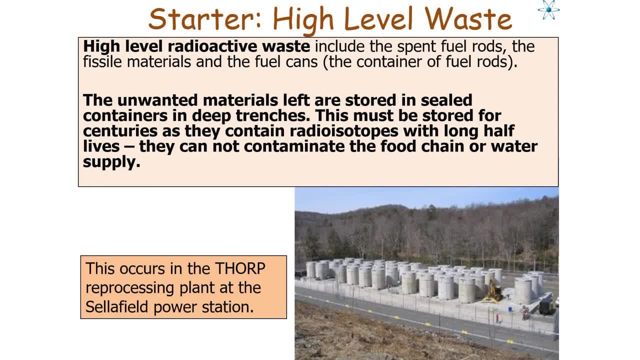 plant. After reprocessing the welded radioisotopes, the sugar particles are reused for plants and then stored in sealed containers in deep trenches. and this must be stored for centuries because they contain radioisotopes with long half-lives so they can't contaminate the food. 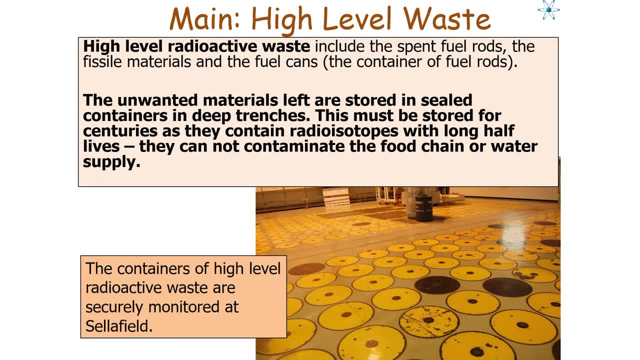 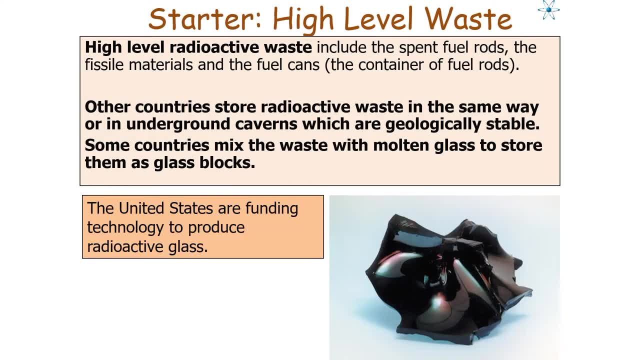 chain or the water supply. So in the UK containers of high level radioactive waste are securely monitored at the Sellafield nuclear complex. So these containers of waste can only be accessed by workers at Sellafield which are geologically stable. Now some countries, such as the United States, mix the waste with 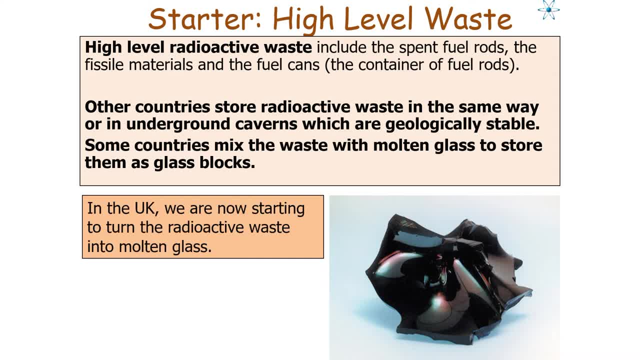 molten glass to store them as glass blocks. Now in the UK we're now starting to turn our radioactive waste into molten glass. Now the process of turning a substance into glass is called vitrification. Now it's safer to keep our radioactive waste vitrified or as molten glass. 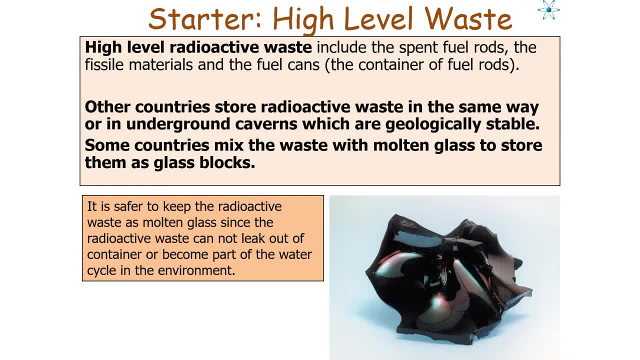 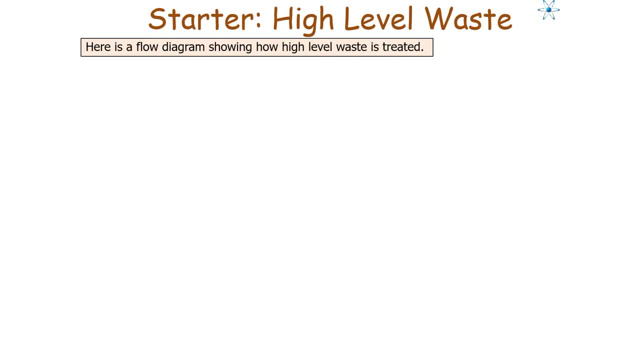 since the radioactive waste cannot leak out of the container or become part of the water cycle in the environment. So here's a flow diagram showing how high level waste is treated in the UK. In stage one, the material is removed remotely. Stage two: the material is cooled underwater for. 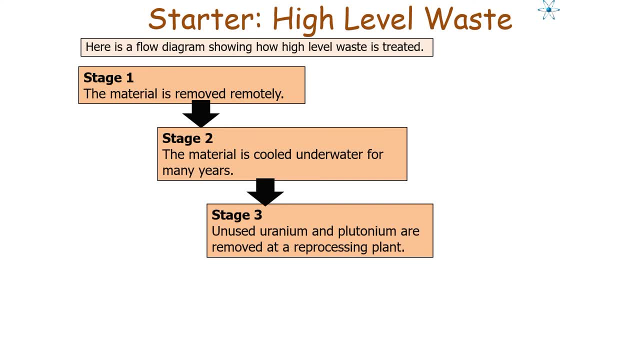 many years. Stage three: unused uranium and plutonium are removed at a reprocessing plant. Stage four: the remaining material is placed in a sealed container and then buried deep underground in a secure location. The material can be turned into glass to ensure there's no leakage in the 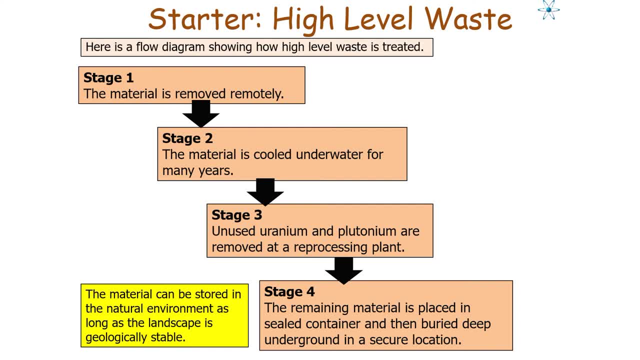 future and the material can be stored in a sealed container. So here's a flow diagram showing how high level waste can be stored in a natural environment, as long as the landscape is geologically stable. So we can summarize our radioactive waste and safety protocols with. 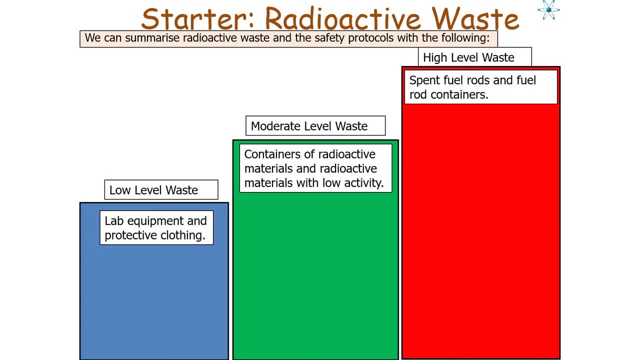 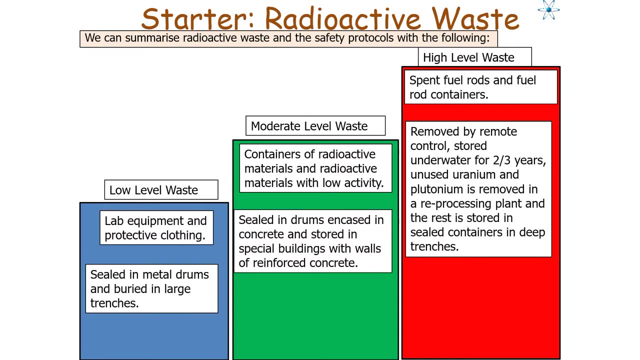 the following: Low level waste is lab equipment and protective clothing. Moderate level or intermediate level waste is containers of radioactive materials and radioactive materials with low activity, whilst high level waste is spent fuel rods in fuel rod containers. So for low level waste, we seal them in metal drums and bury them in large trenches. For moderate level, 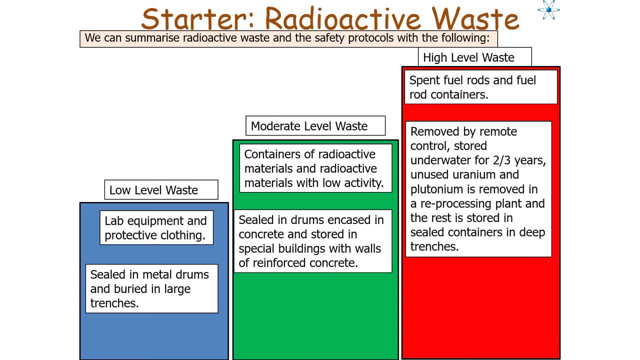 we seal them in drums encased in concrete and stored in special buildings with walls of enforced concrete. Whilst for high level air waste, we remove them by remote control, store them underwater for two or three years. any unused uranium and plutonium is removed in a reprocessing. 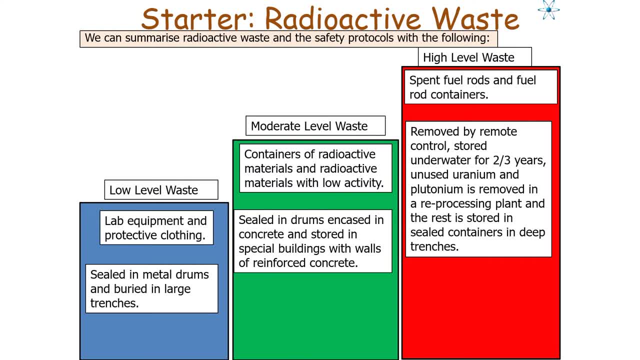 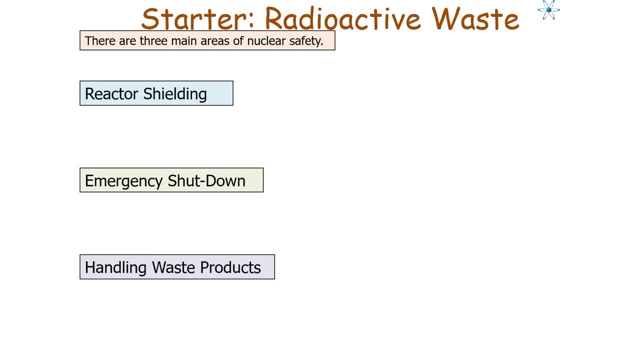 plant and the rest is stored in sealed containers and deep trenches. So if we consider our three areas of nuclear safety, Well, firstly, we have reactor shielding. So reactor shielding is that when a nuclear reactor is surrounded by thick concrete, it'll act as a shield. This prevents any 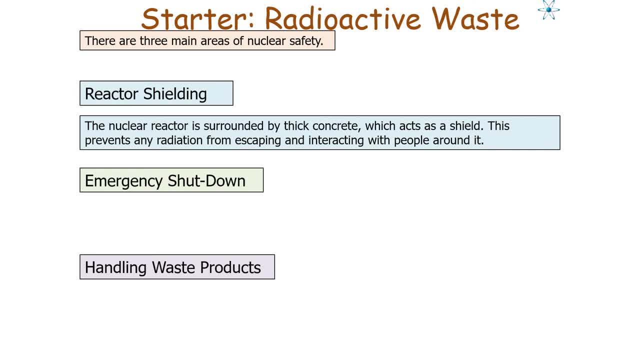 radiation from escaping and interacting with people around it. You've also got the emergency shutdown procedure in a nuclear reactor. So in an emergency the nuclear reactor can be shut down by releasing the controls fully into the reactor. This will slow down the fission process as quickly. 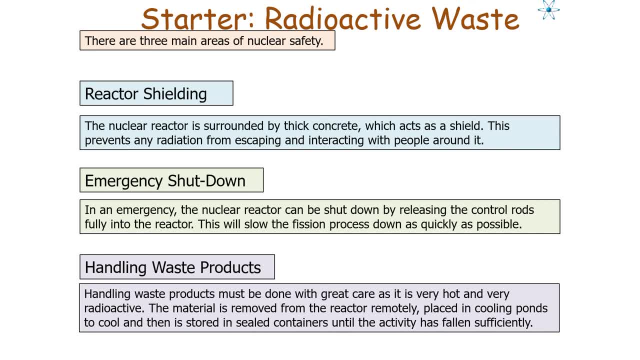 as possible. And finally you've got handling waste products. So you've got to handle the waste products with great care, because it's very hot and very radioactive. The material is removed from the reactor, remotely placed into cooling ponds to cool and then is stored in sealed containers until the activity has fallen sufficiently. 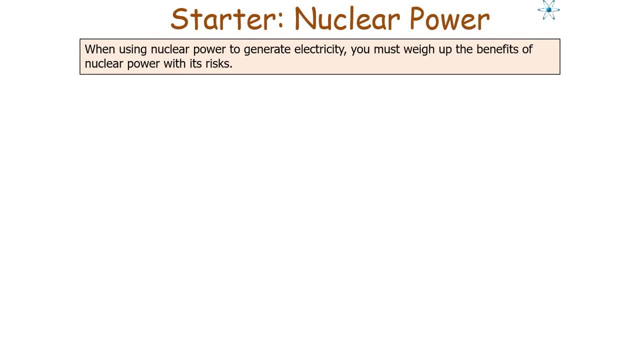 Now, when we use nuclear power to generate electricity, we've got to weigh up the benefits of nuclear power along with its risks. So what are our benefits of nuclear power? Well, firstly, we can say that there's a lot of nuclear fuel allowing us to use nuclear power. 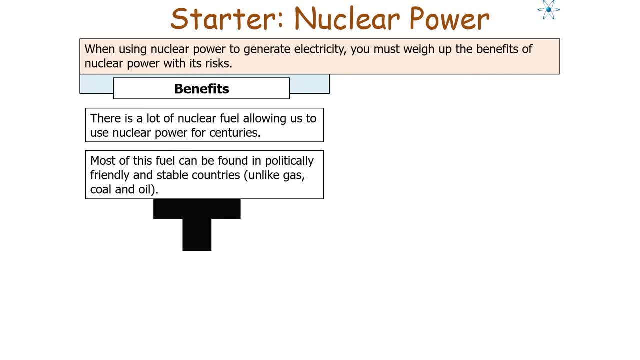